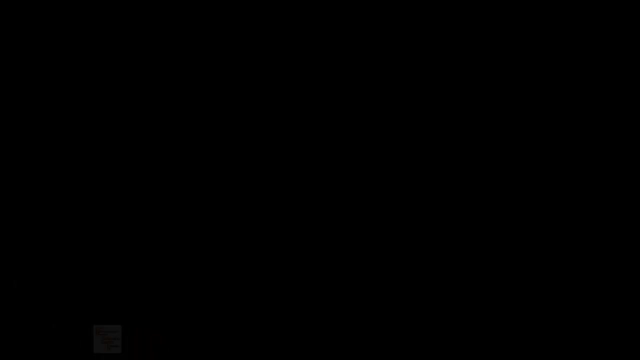 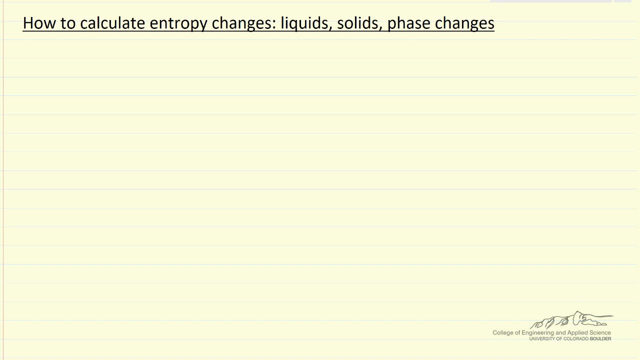 Here we're going to look at how to calculate entropy changes if we have a liquid or solid, temperature changes or if we go through a phase change from, say, a liquid to a gas. And the way we're going to do this is to start with our definition of entropy change, which 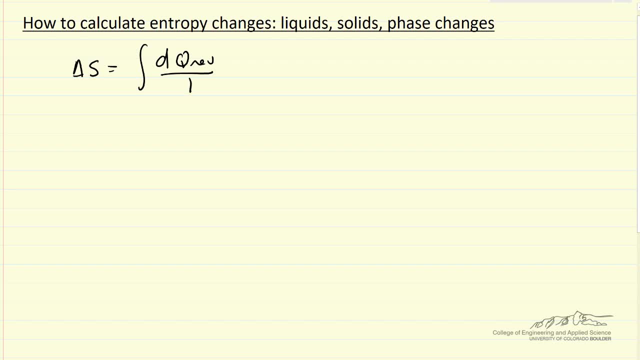 is the integral dq reversible over T, where T is absolute temperature. The idea is, if we're at state one and we go to state two, if we pick a reversible pathway and then the heat transfer at any point divided by the temperature, at that point integrated. 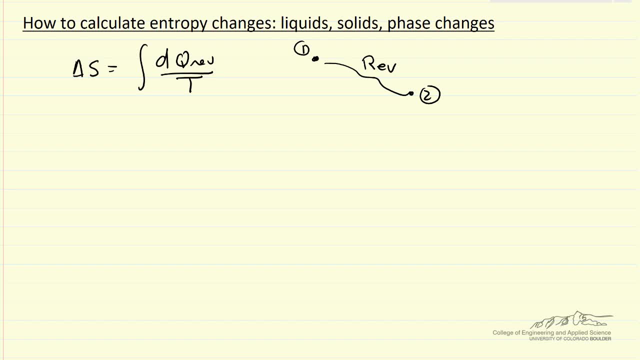 gives us the entropy change, And so to get the heat transfer we're going to use the first law. so let me write down the differential form, The first law for a closed system, so Q reversible and work reversible. So work reversible would mean pressure times differential. 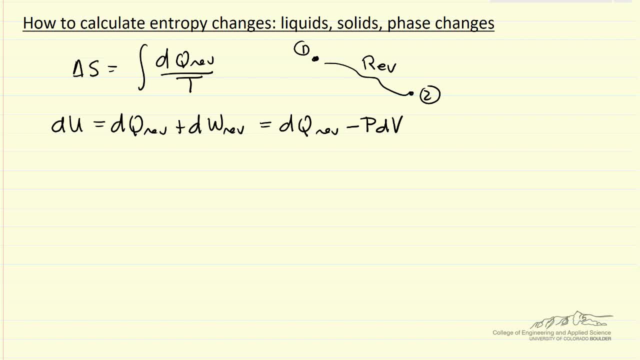 Now it turns out, changing pressure has very little effect on a liquid or a solid. We don't change the enthalpy, we don't change the entropy, we don't change the volume, etc. So to first approximate For a liquid solid we can write this as minus the differential of PV. 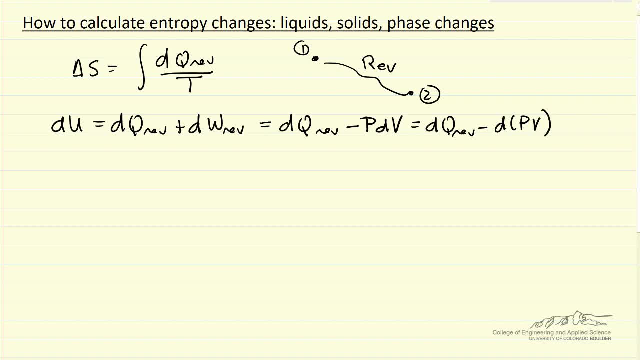 Now what I'm going to do is take this term, bring it to the other side of the equation and we'll see that we have, on the left, du plus dPV and u plus PV is h. so this is dh, is dq, reversible. 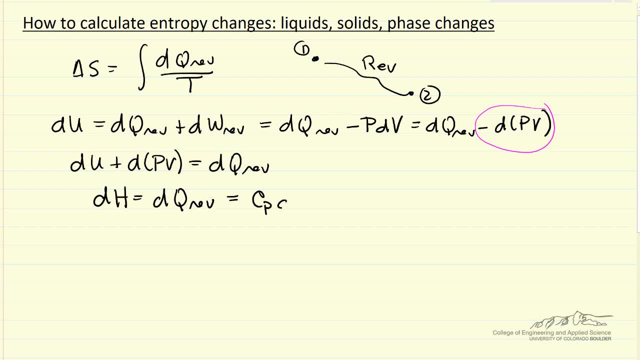 dh For a liquid or solid is heat capacity Cp times dt. So that means, if we now want to calculate the entropy change and again let's rewrite our definition and dq reversible is Cp dt over T. Heat capacity for liquid or solid does not change much with temperature, some reasonable.